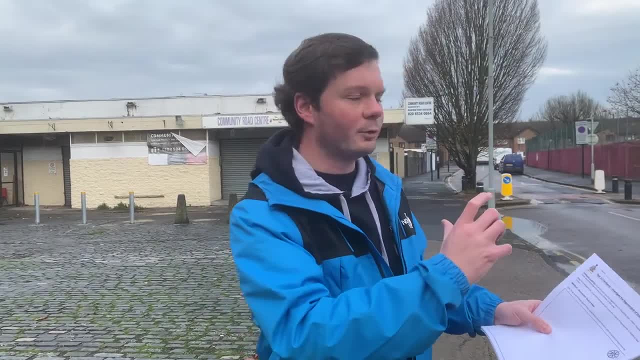 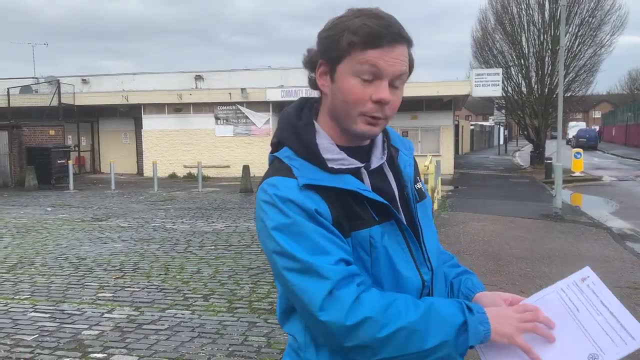 field sketch, and why do we bother doing that? Taking a photo is great. you can get a really good idea of what the area looks like, but you can't annotate it whilst you're there. So if you're drawing a field sketch here, say, for example, we're drawing a field sketch looking 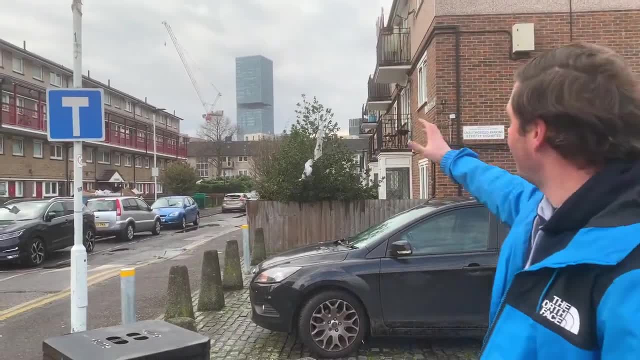 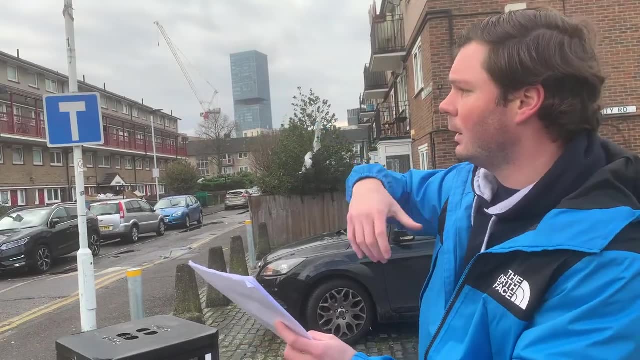 here we've got in the background we can see. here we've got Stratford, we've got the regeneration, we've got cranes. you would draw here where we've got our homes, here, looking at the quality, the building quality of the homes, then we would have. 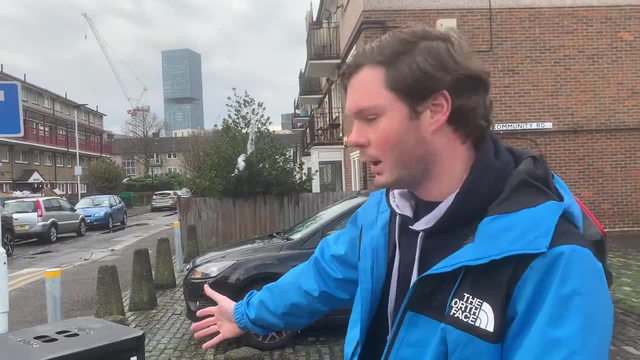 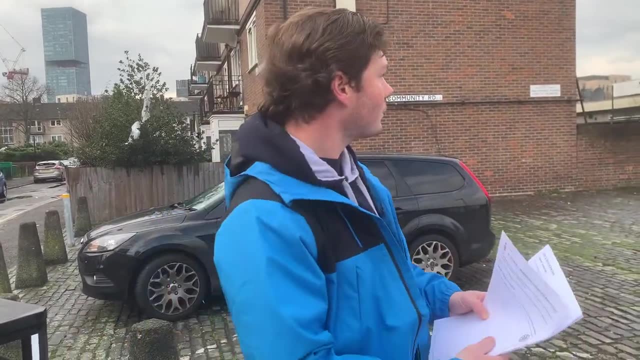 the cranes in the background showing the regeneration in the area. We're looking at bins. it's important to see environmental quality of the area. is there bins? is there sanitation in the area? Looking at our places boarded up as an example and you would draw that and annotate- 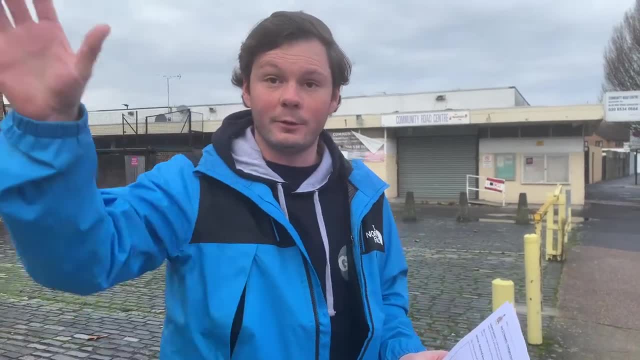 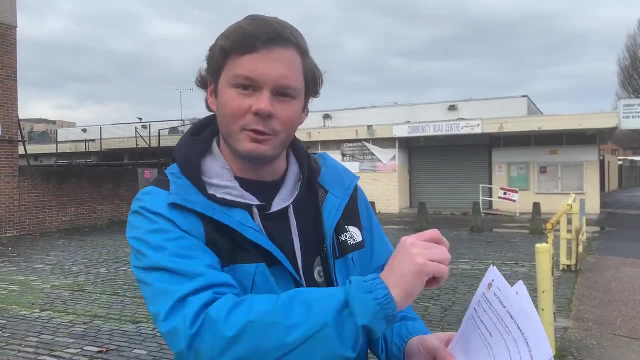 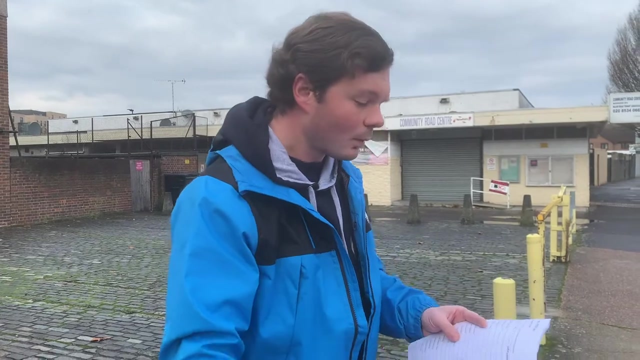 that on your field sketch. Now you would do this all three sites so that you've got a good and clear representation of the area here. It's important make annotations, take notes when you're doing that, because then you get a good flavour as to what life is like here in Stratford, The next one we can look at. 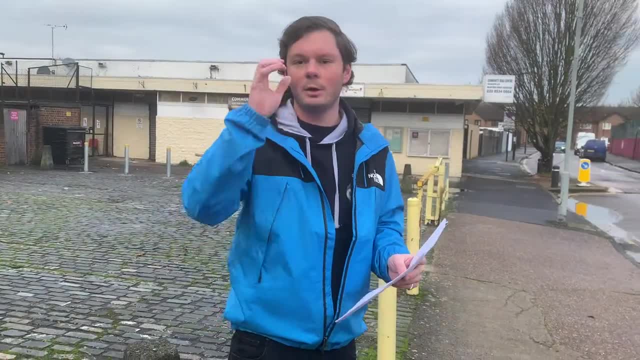 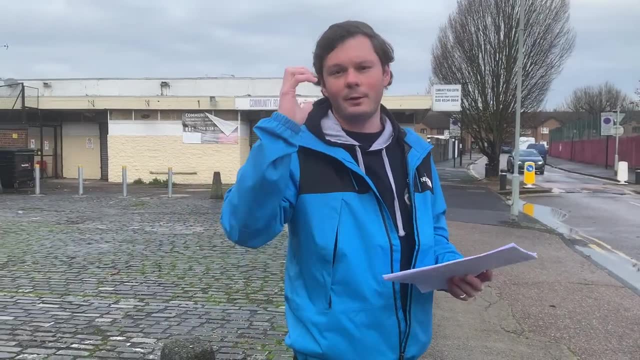 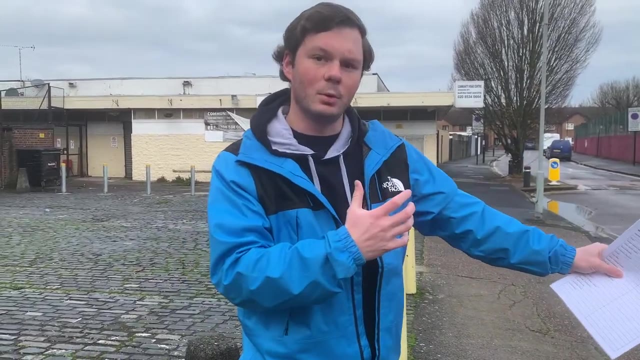 is this idea of a service tally? Now this brings me on to looking at the concept of quantitative versus qualitative data collection methods. Qualitative data collection is looking at interviewing people. So in this instance, if we were to interview people, you would get an opinion based argument. 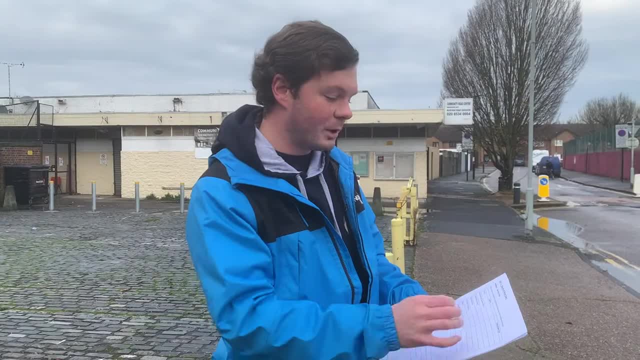 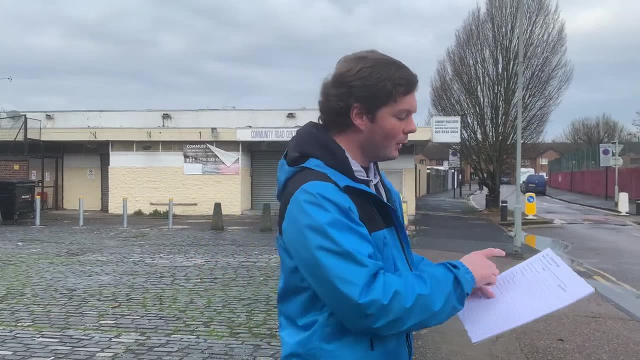 but then if you're wanting quantitative, that is, numbers, so we could do here and we've got here a service tally. so we're trying to work out what the service is in the area. So when we're at our chosen sites we'll tick off: right, we've got a school here, tick, can we see any? 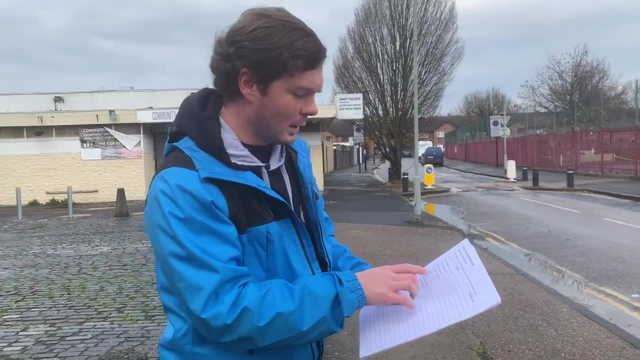 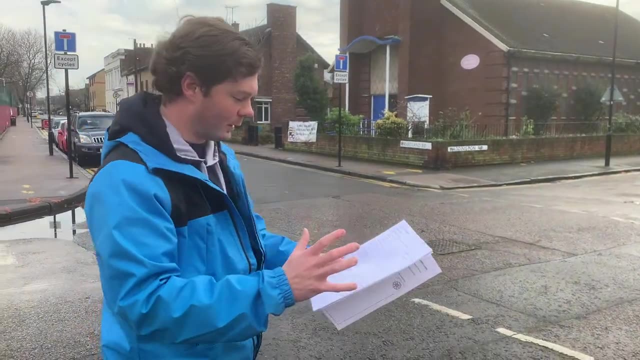 leisure centres or sports venues? no, not that I can see. can we see a place of worship? yes, behind us here we've got a place of worship. I'm going to tick that off. is there a library? not that I can see. health and beauty, a pub? 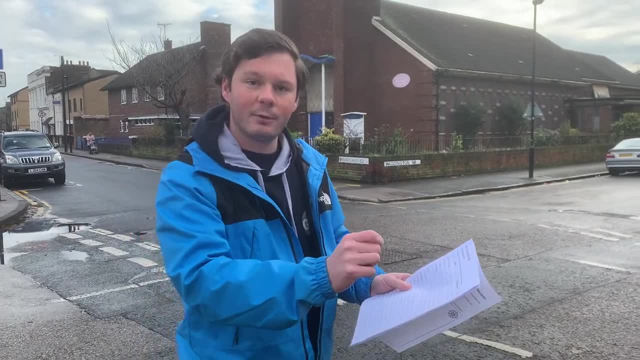 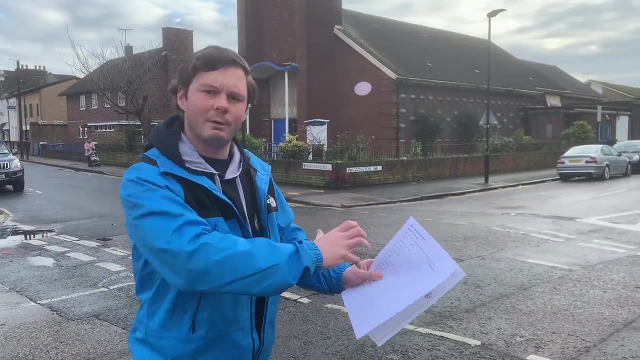 estate agent. what have you? and you start to tick off these different services as you go, this being quantitative data collection methods. you'll do this at your three sites to be able to see what are the services at each of your chosen sites. Then, when we move on to our 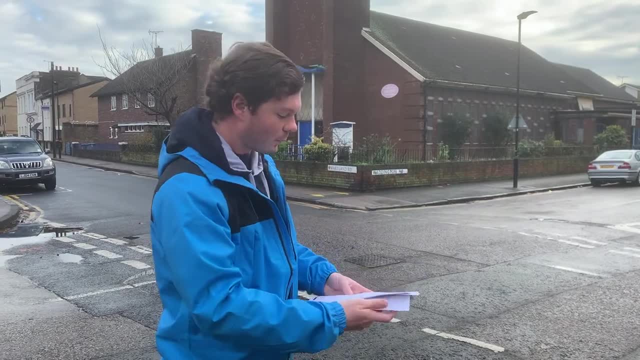 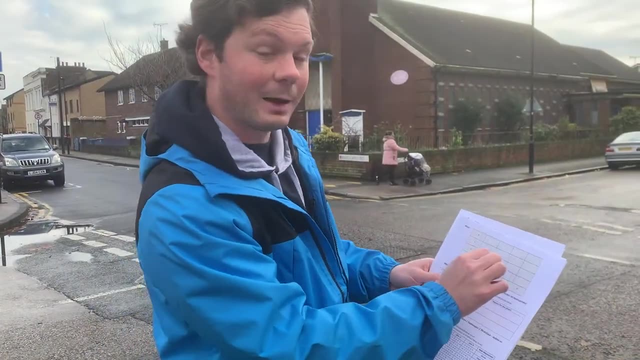 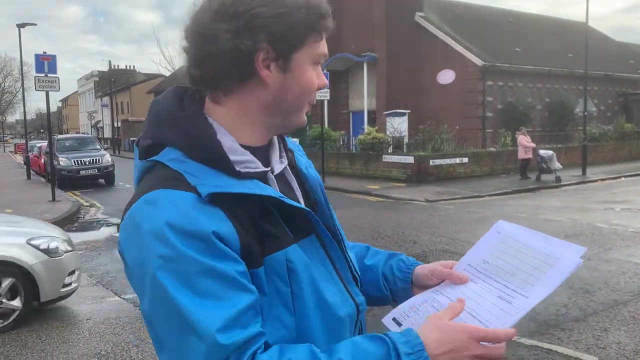 next section. we've got here. we've got here- a map showing where we are. so I want students to be able to start to plot on a map exactly where we are, what are our three sites, so that we can really start to point out where in this area are we collecting data. Then what we can start to do is take photographs. 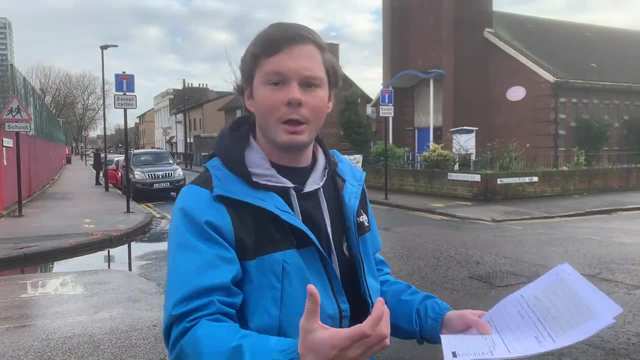 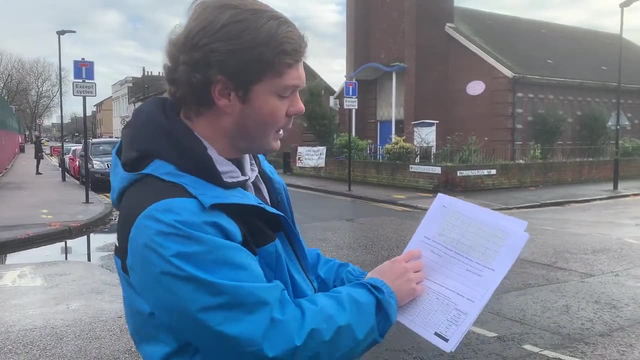 it's really important to take images so you can get a clear picture as to what life is like, so that when you're back in the classroom you're able to see what it was like when you're there. So here you would take a photograph and then you take notes on your location. why? 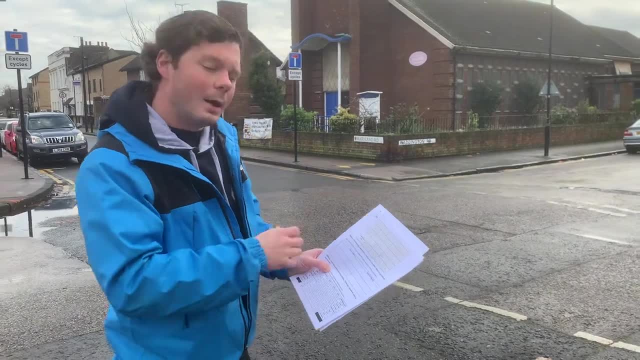 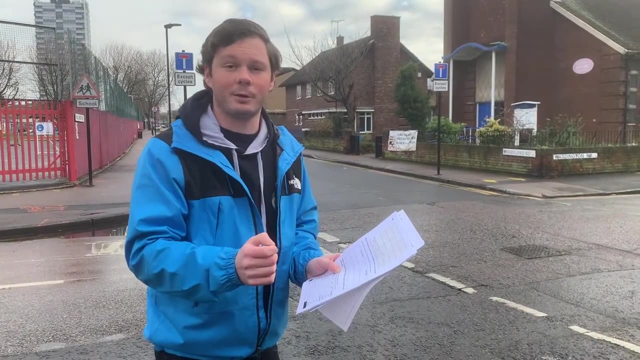 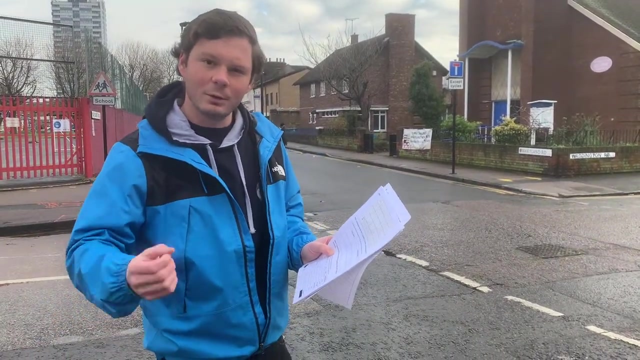 you chose to take that photograph, Have you. every time we do this, it's important you state if you're taking a random, systematic, systematic or stratified sampling strategy. it's really important so that you know exactly what you've done and to be consistent throughout this process to make your data as accurate. 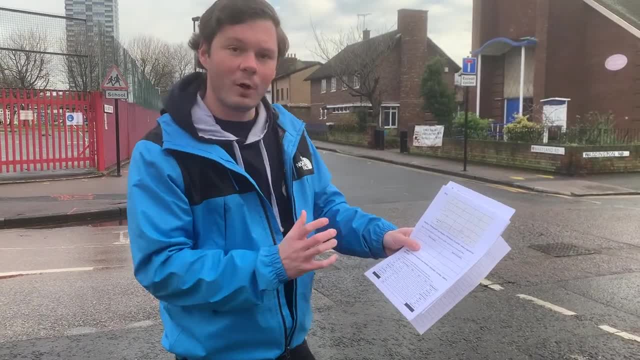 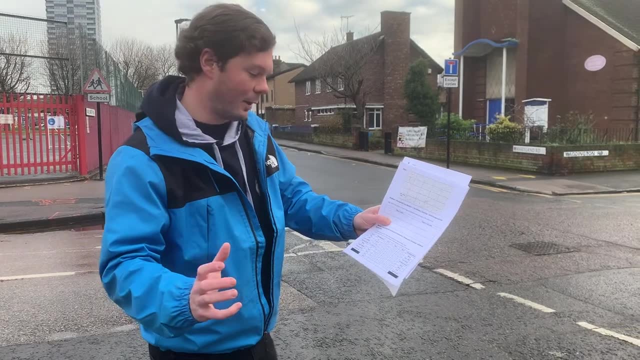 as possible. We then have what we call an environmental quality survey. an environmental quality survey is a really good way to see what the environmental quality is for the area, and you'll notice we've got A lot of factors, so the first one could be litter on one side of the survey you've got. 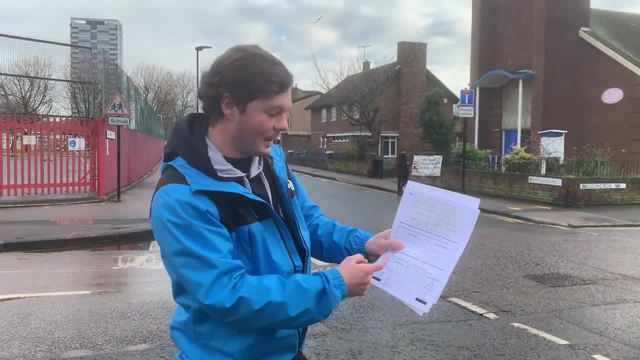 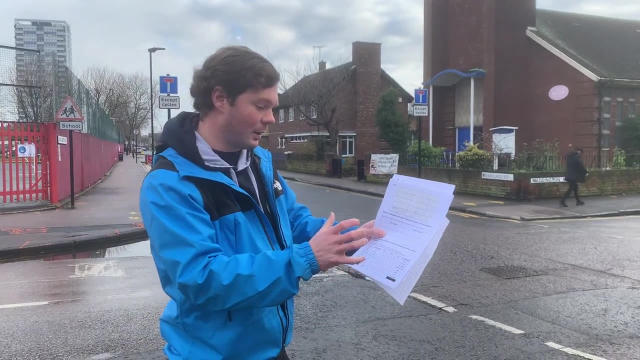 there's lots of litter, the other side there's none. and at each of your three chosen sites you can do one, two, three, four or five and you state: if you think that there's a lot of litter, that'll be a five, or if there's not much litter, there's a one, but there's. 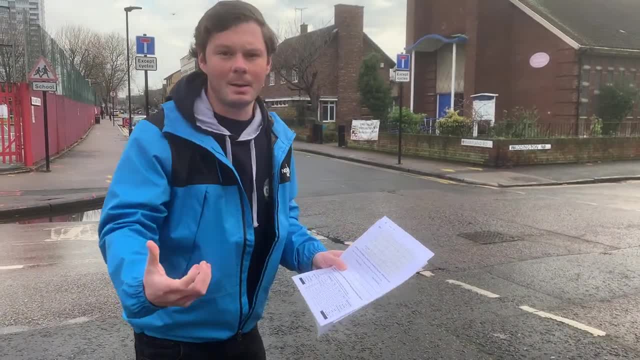 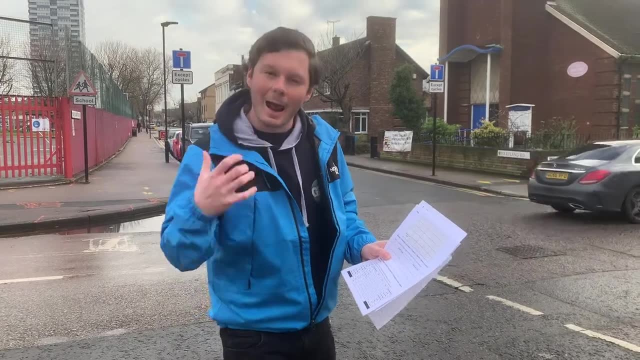 a problem with this data collection method. this is very opinion based. okay, it's subjective, it's your own personal opinion of that area. So to what extent is that an aspect of your data collection? So to what extent is that an aspect of your data collection? 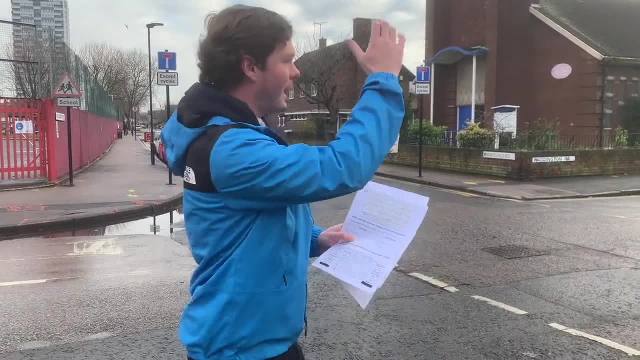 Well, if you are collecting data, You know you can do the left hand side and then use the right hand side to collect the data from each site. So you know that is extremely important. So you're currently collecting data, which is particularly important because you're 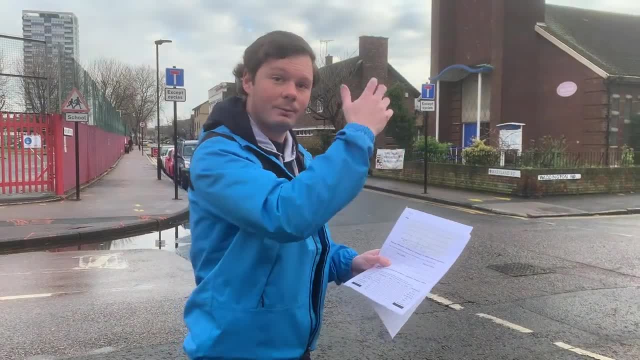 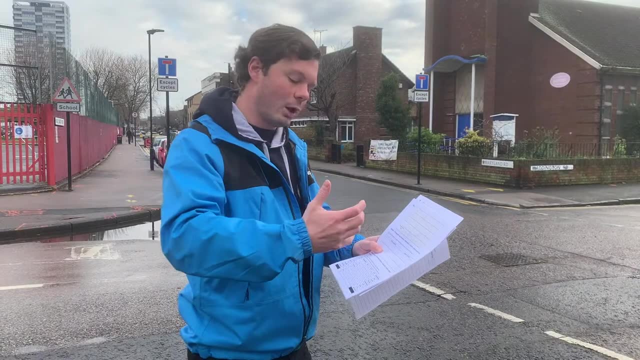 relatively secure when collecting data. But then if you do that at each site, so you've got three different sites. you do that at each site and you do that three times- Stratford New Town, East Village and also Hackney Wick- you start to collect data that is quite reliable as you're doing it at different range of sites. 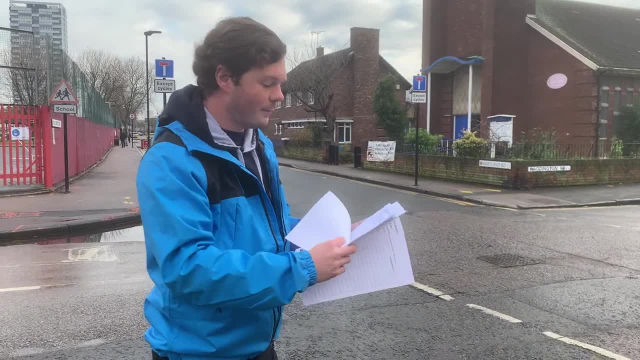 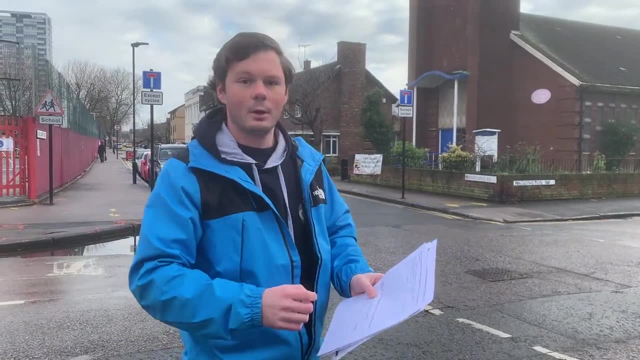 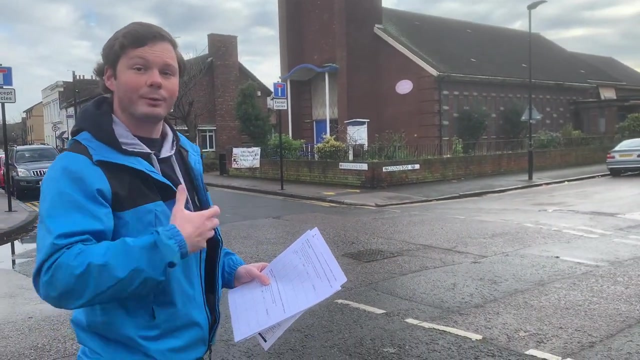 so it's a good way to collect data. On top of this, you can also collect more quantitative data collection, that being a pedestrian count. So for one minute- And you might be looking in this direction- for one minute You're going to count up how many people do you see? 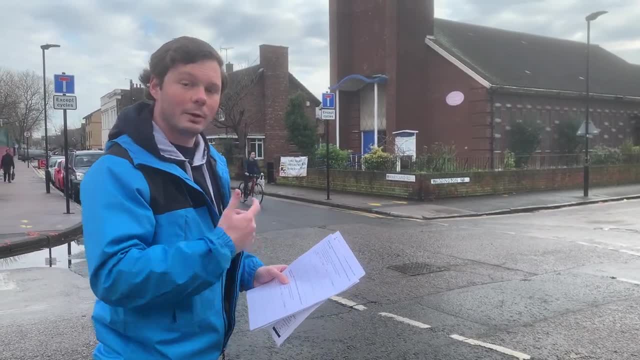 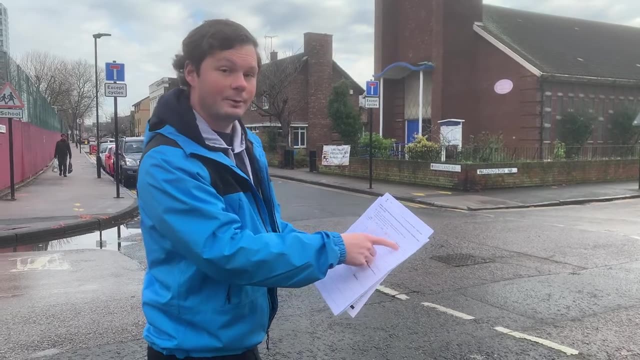 Once you've done that, you'll do this three times, Three times, and you'll do that for a minute. to make it consistent and to collect as much data as possible, You can also note down how many people did you see? Why do you think there aren't that many people here? 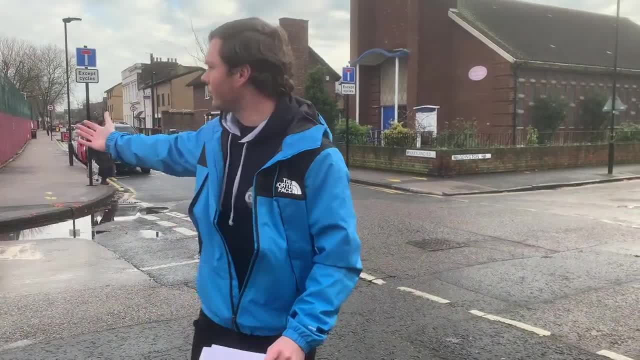 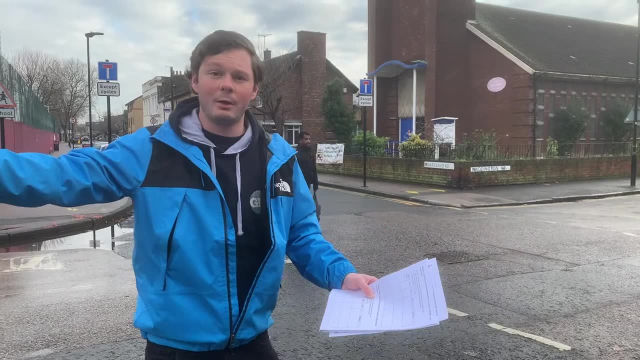 As an example, today we're here on a Sunday. The school isn't open, so it's very quiet. Obviously, we're in the middle of a lockdown, which means that people won't be out. The community centre here is shut. 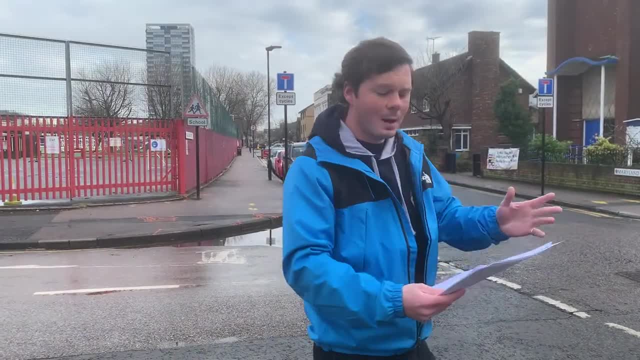 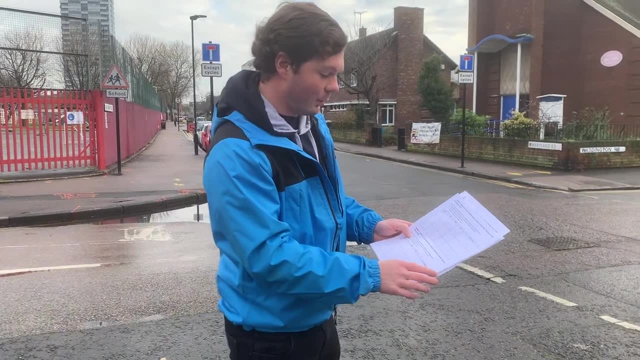 Not many people are out and about. what have you? Making it very different to what it might be like on a Tuesday morning at, say, 10 o'clock. And finally, we also have what's called a traffic count. So you count the number of cars you see in the area. exactly the same method. 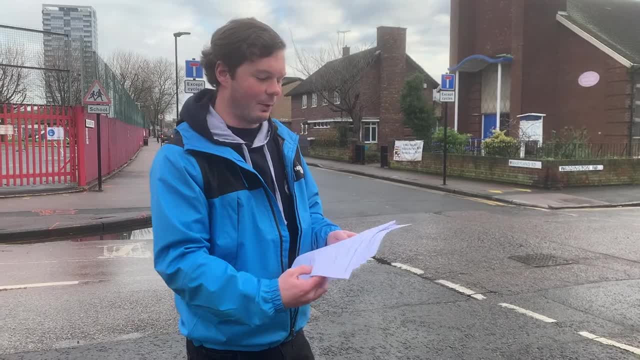 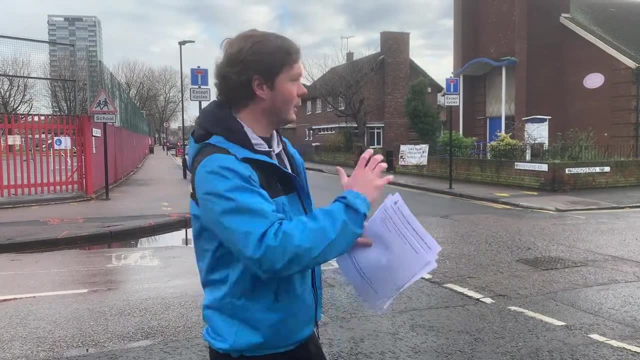 to start to see what the environmental quality is like in that area. So we've got here. then There's a range of strategies that you can use, and you'd do this at site one just down here, 100 metres away here. 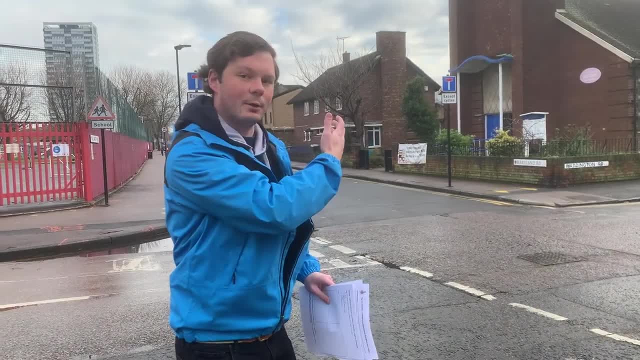 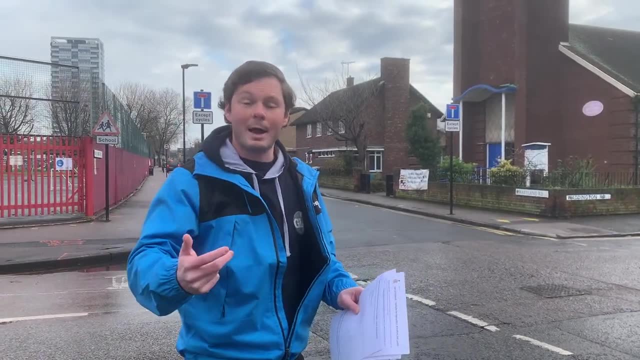 at site two here and then site three 100 metres down in that direction, And you'd use a range of sampling strategies- random, systematic and stratified- And with that you collect it three times. try and get as much data as possible. 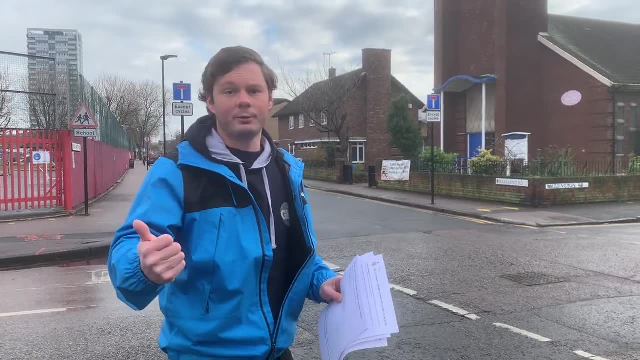 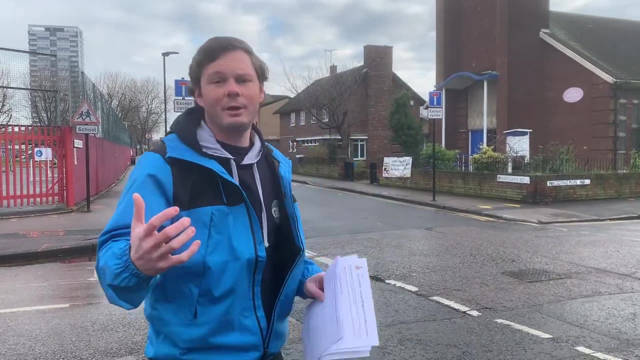 to try and make your data as accurate and reliable as possible at this chosen site. So we're going to be moving on to our next site, looking at East Village, where the Olympic Village is to start, to see how does the regeneration change from here. 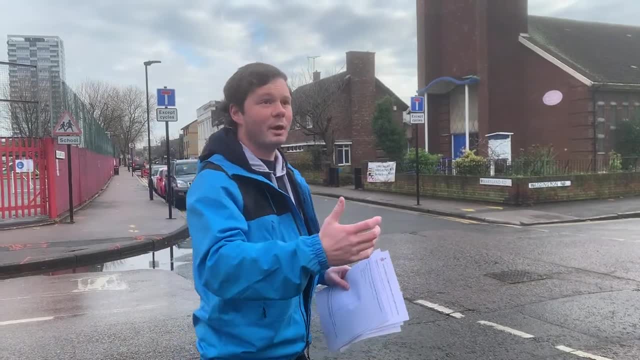 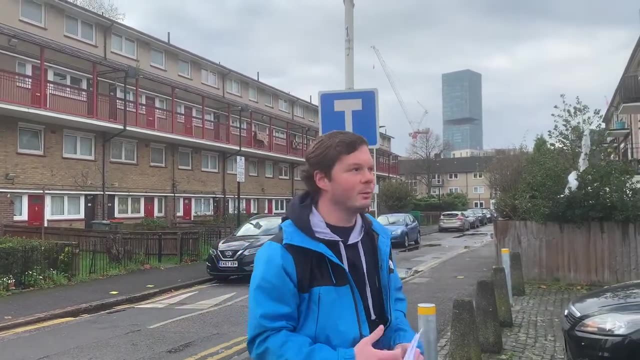 where we are in very much a residential area, not much regeneration, as you can see behind us. We've got here, we can see the skyscrapers, the more modern idea of the regeneration, And we'll start to think about why is it that this area is very different to an area like that.